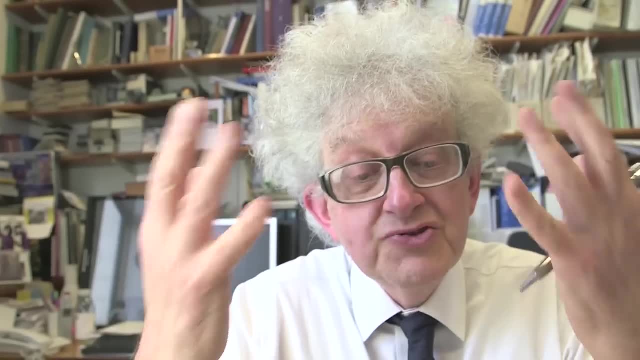 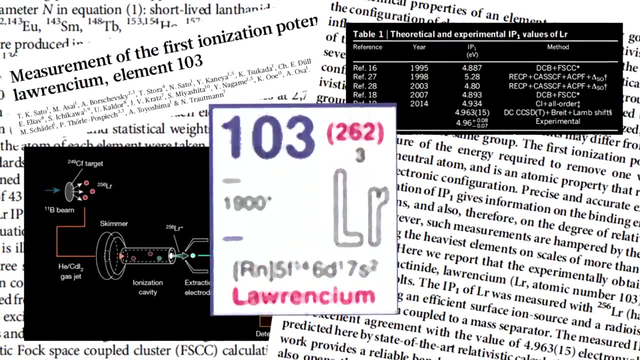 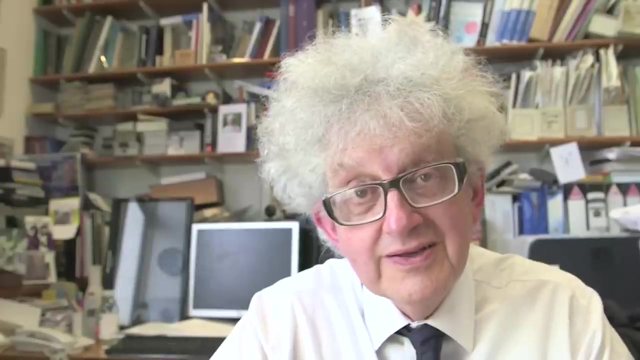 at the end. here is, experimentally, a triumph. Lorentzium is a so-called super heavy element. You have to synthesize it in accelerators. It has a very short half-life. The isotope they were measuring has a half-life of 27 seconds. 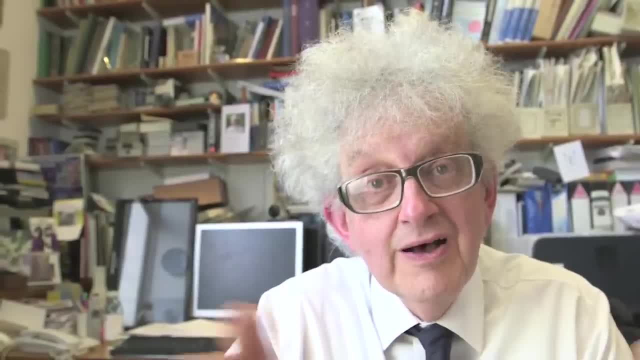 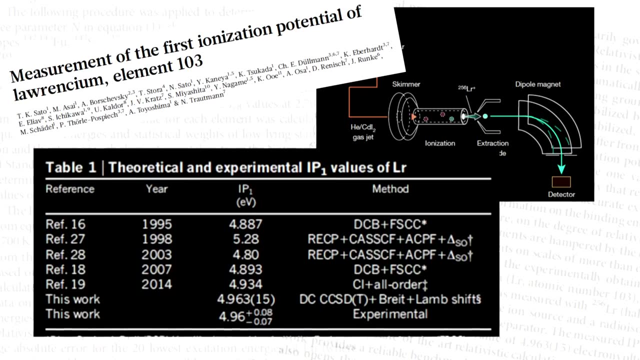 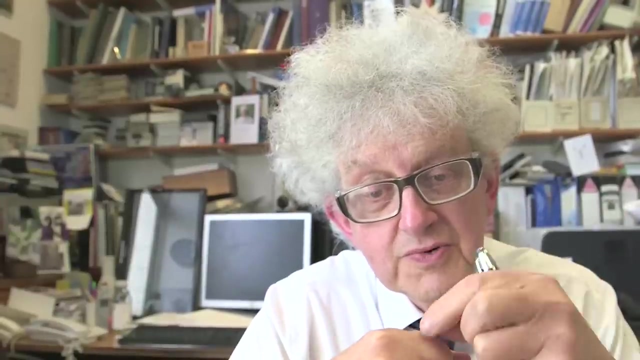 That means after 27 seconds half your Lorentzium is gone. And they were doing measurements on individual atoms And they were measuring a slightly obscure quantity, the so-called first ionization energy, which is the amount of energy you require to remove the first electron. 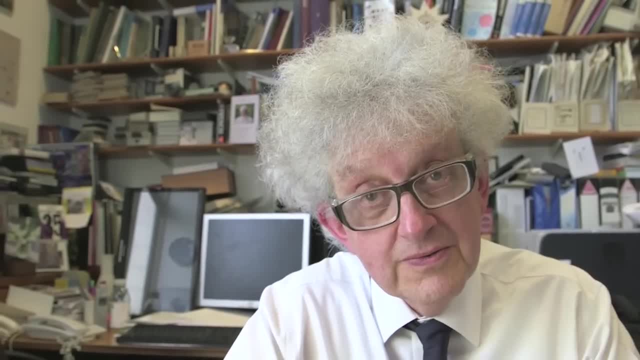 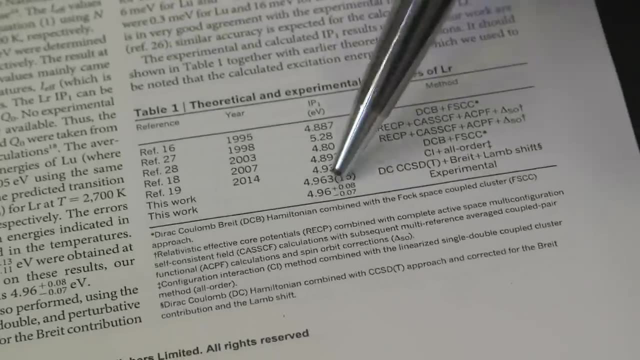 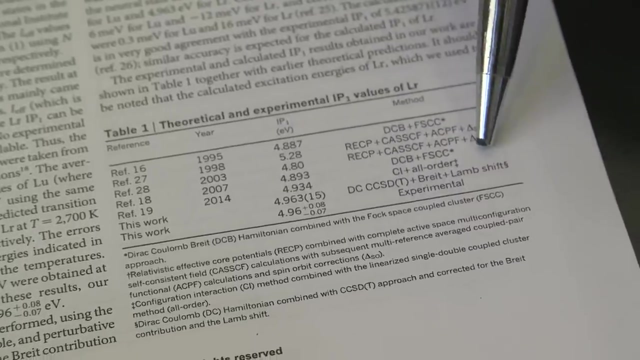 And what they discovered was that Lorentzium has a very low first ionization energy And quite pleasingly, you can see that the value that has been measured, 4.96 electron volts, is almost identical to what has been calculated by theory. But what's this got to do with the periodic table? What they're? 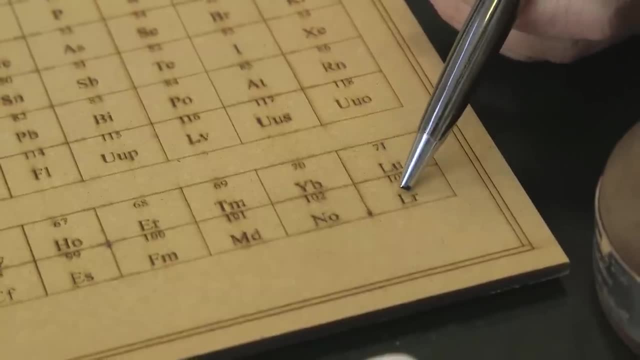 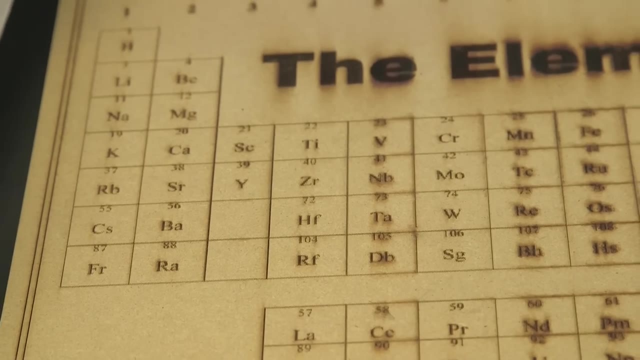 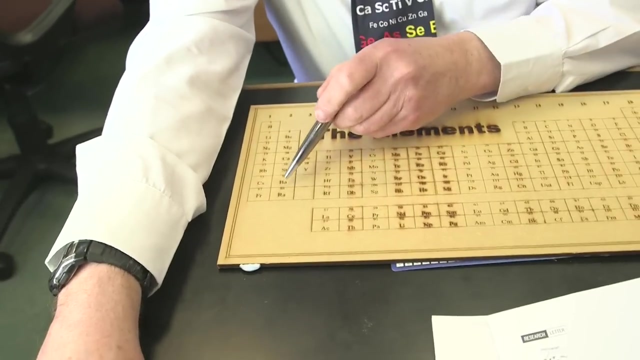 suggesting is that lutetium and Lorentzium should be sitting under scandium and yttrium. The big break in the periodic table should actually come there rather than there. So if you have the short form, you would have the dot over radium. you'd go down to actinium. 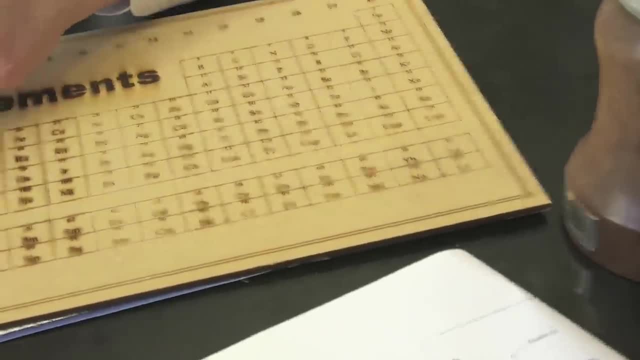 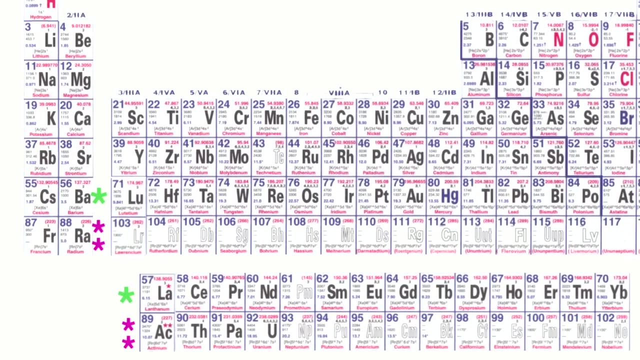 you'd go along to nobilium and then up here to Lorentzium. So what they're saying is that the properties of Lorentzium are much more like yttrium and scandium than the properties of lantium. So what they're saying is that the properties of lantium and lantium are much more like lantium and actinium than the properties of lantium and actinium are. 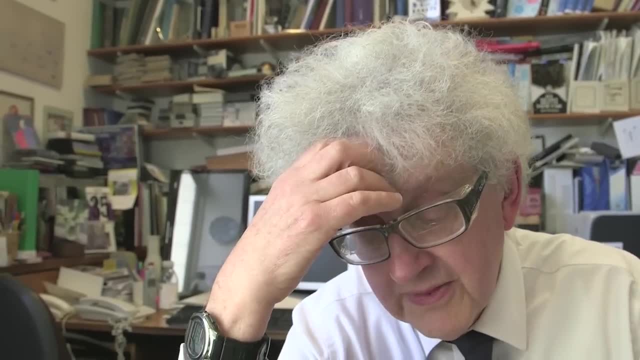 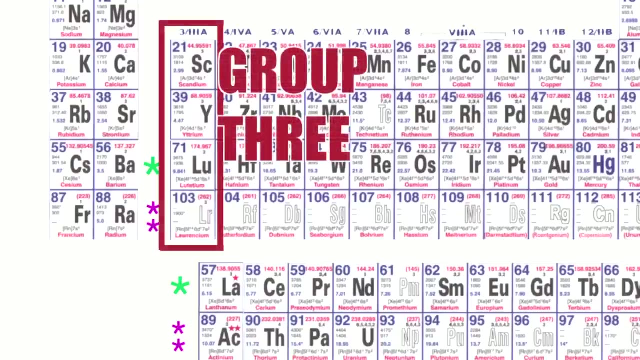 Their argument is that the ionization energies of Lorentzium fit much better with those of this group than the ionizations of lantium and actinium do. So what they are saying bluntly is: lantium and actinium probably shouldn't be in group three. Lutetium and Lorentzium should be in group three because